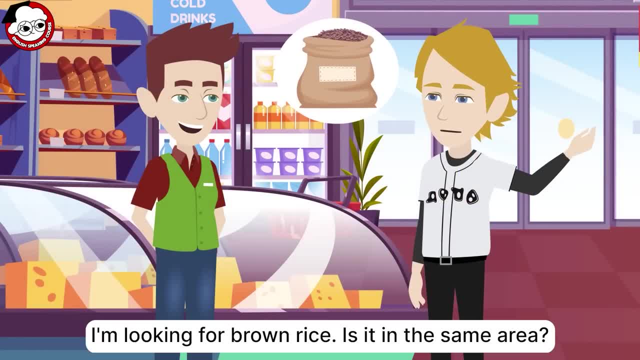 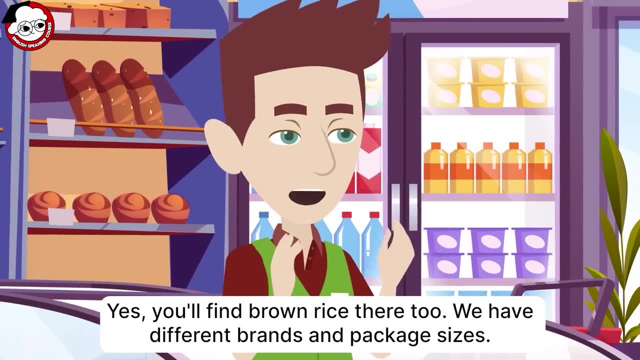 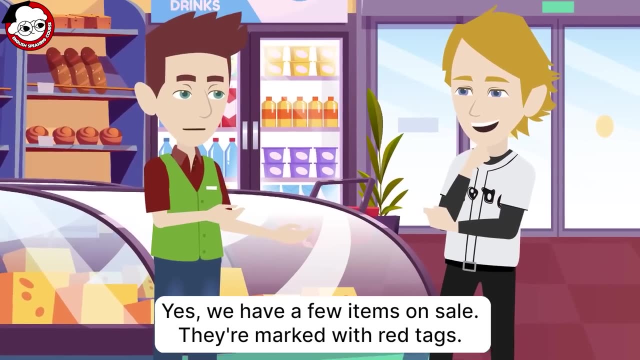 Do you need a specific type? I'm looking for brown rice. Is it in the same area? Yes, you'll find brown rice there too. We have different brands and package sizes- Great. Also, do you have any discounts today? Yes, we have a few items on sale. 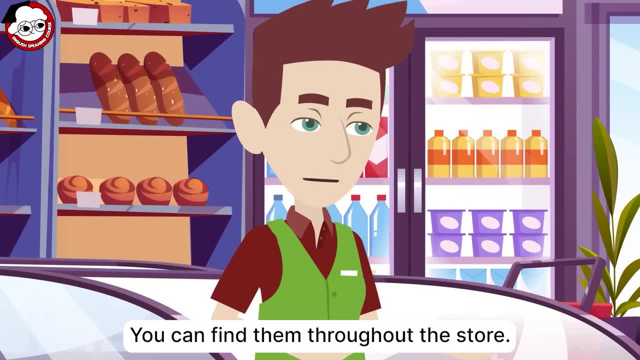 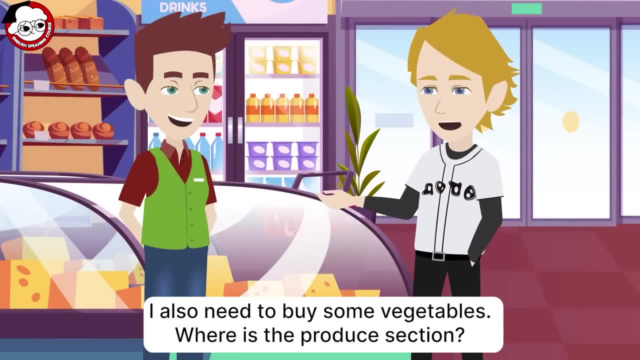 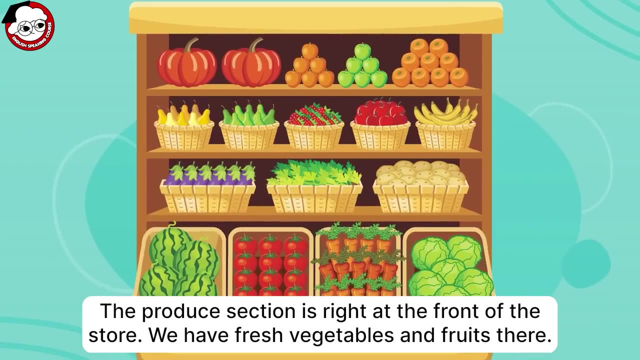 They're marked with red tags. You can find them throughout the store. That's good to know. Thank you, I also need to buy some vegetables. Where's the produce section? The produce section is right at the front of the store. We have fresh vegetables and fruits there. 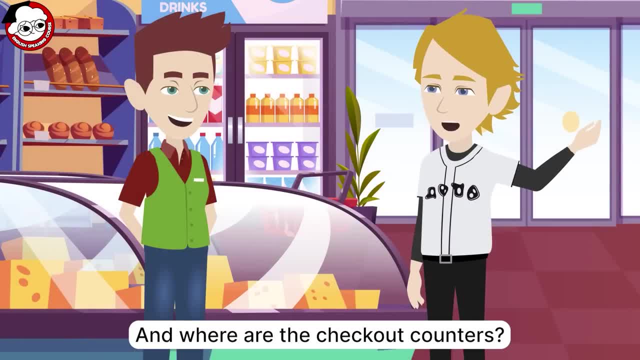 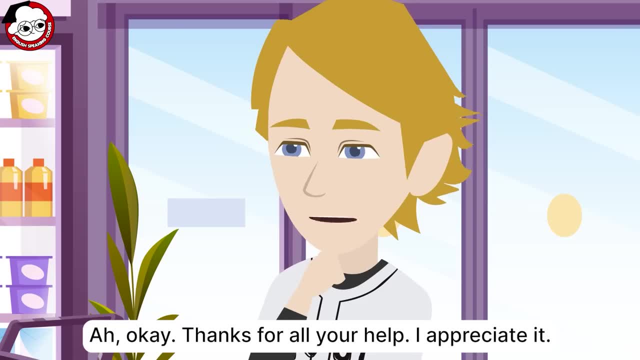 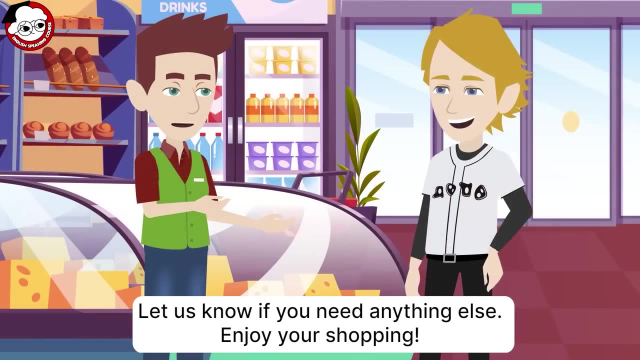 Perfect, I'll check it out. And where are the checkout counters? The checkout counters are near the exit. Ah, okay, Thanks for all your help. I appreciate it. You're welcome. Let us know if you need anything else. Enjoy your shopping. 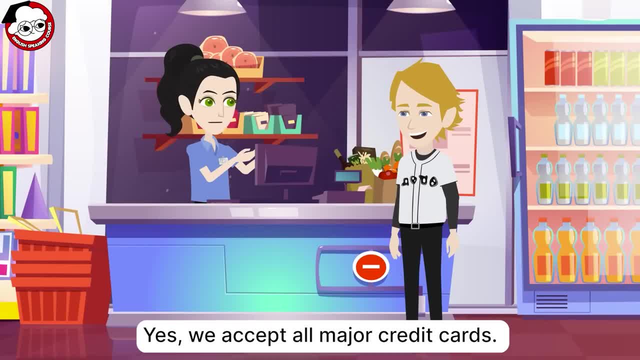 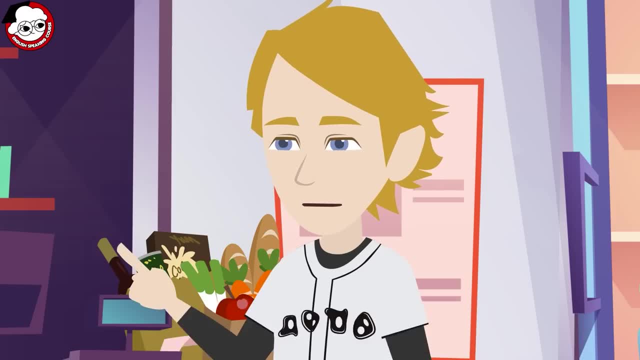 Can I pay with credit card here? Yes, We accept all major credit cards. Great, I also have some coupons. Where should I give them? You can hand them to me. I'll scan them with your items. Here they are. I hope they're still valid. 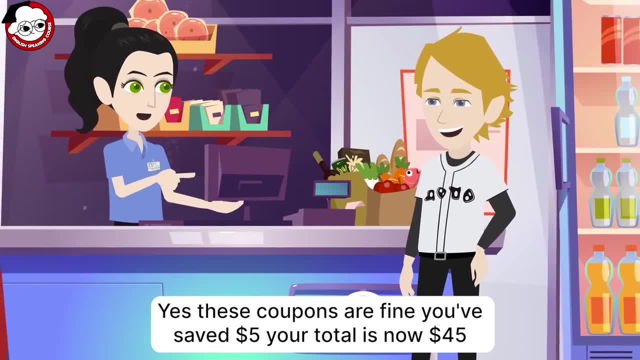 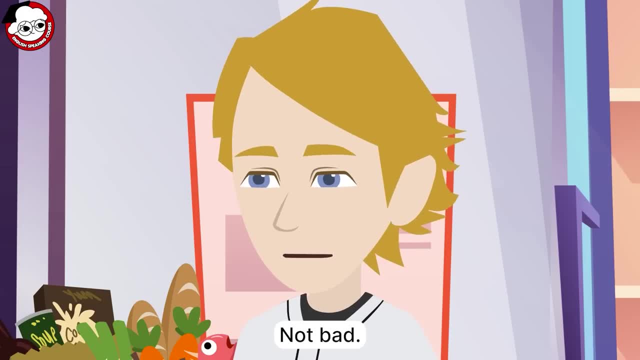 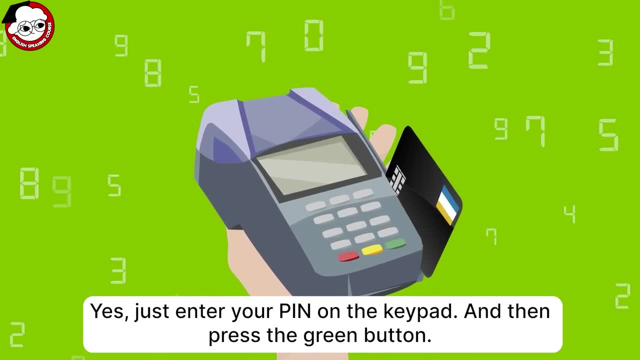 Let's check. Yes, these coupons are fine. You've saved $5.. Your total is now $45.. Not bad. Here's my card. Do I need to enter a PIN? Yes, Just enter your PIN on the keypad and then press the green button. 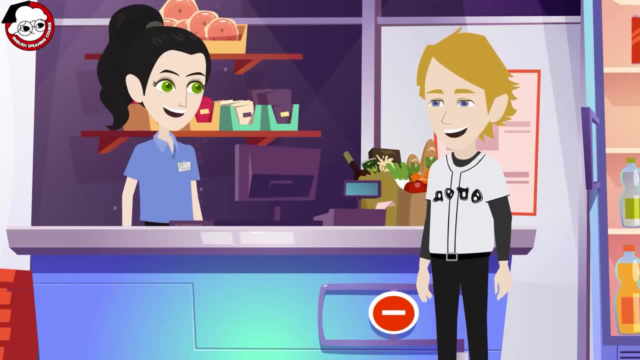 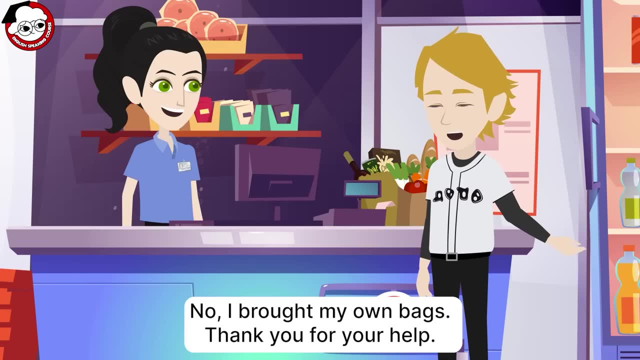 Done. Did it go through? Yes, It's all set. Here's your receipt and your card back. Do you need a bag? No, I brought my own bags. Thank you for your help. You're welcome. Have a great day. 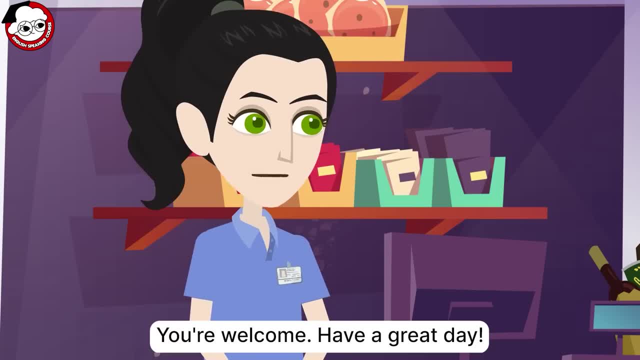 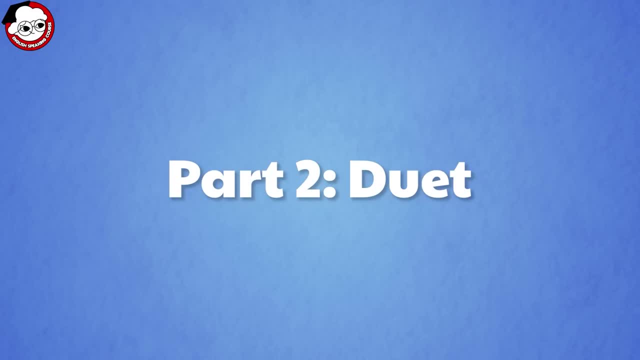 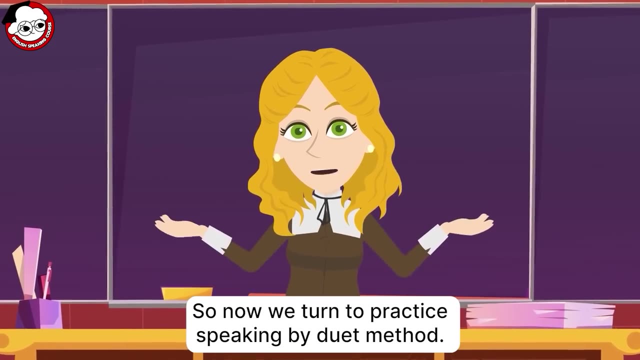 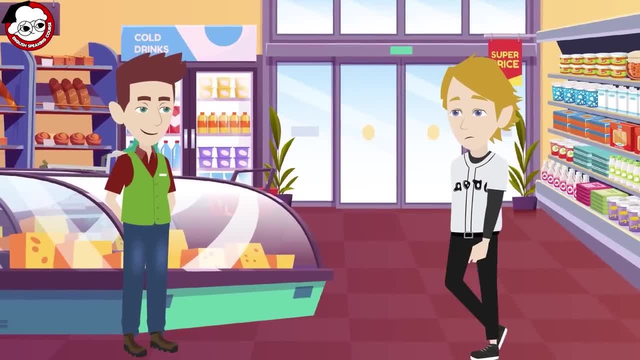 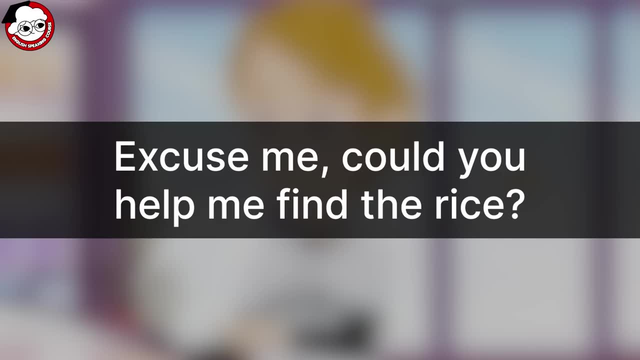 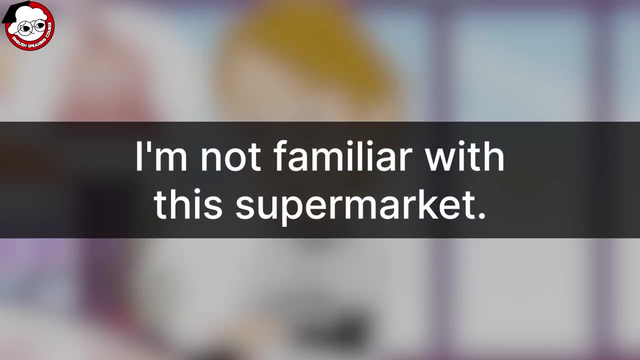 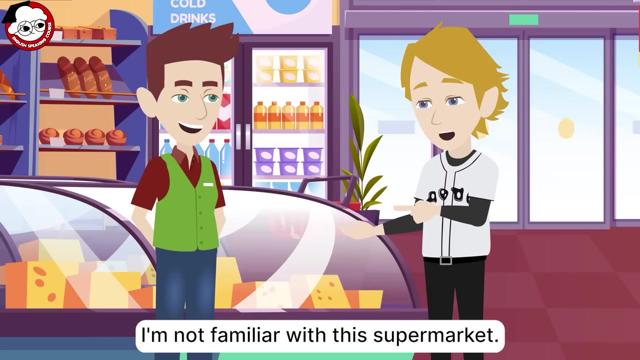 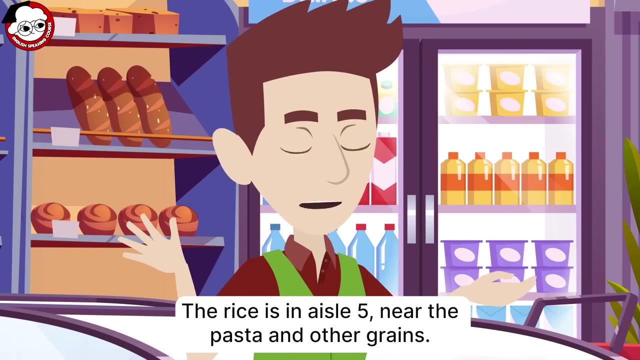 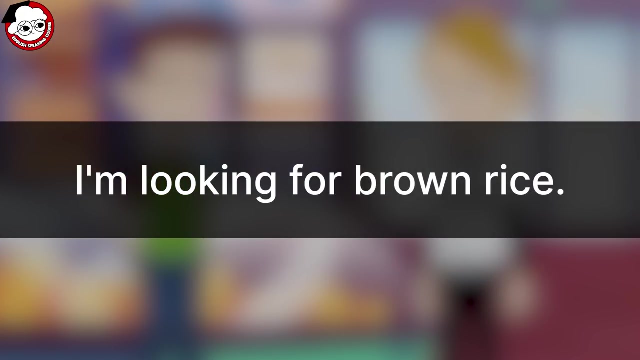 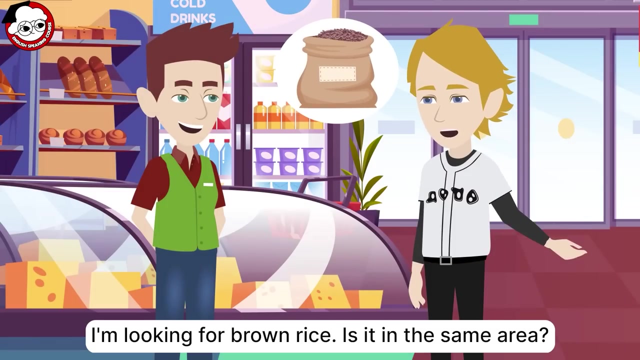 üler lg метimλ. I'm not familiar with this supermarket. Of course, The rice is in aisle 5, near the pasta and other grains. Do you need a specific type? I'm looking for brown rice. Is it in the same area? 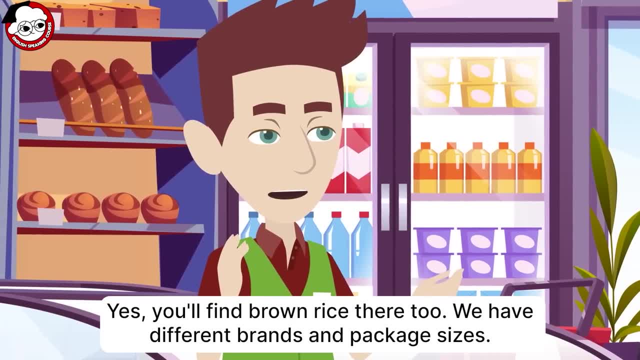 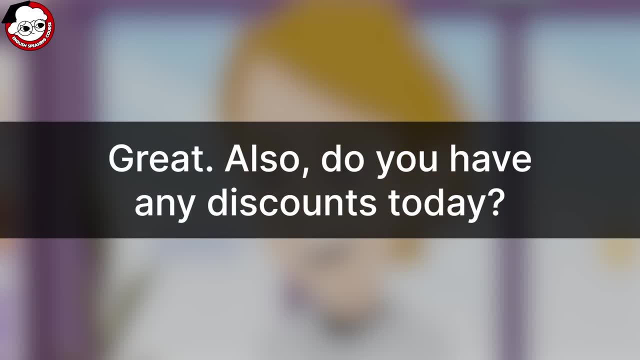 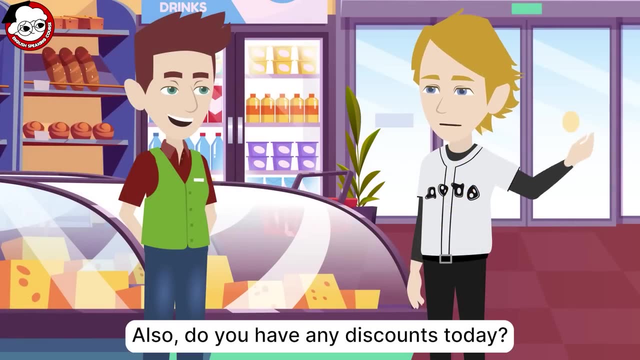 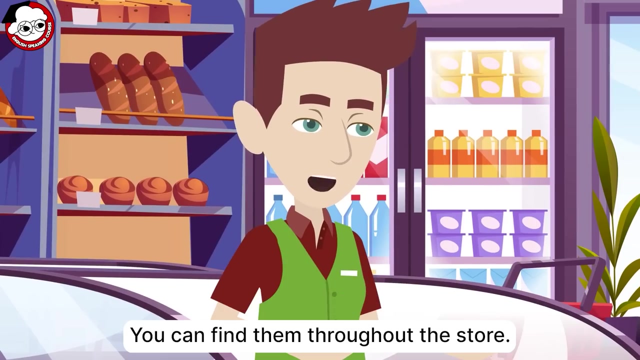 Yes, you'll find brown rice there too. We have different brands and package sizes- Great. Also, do you have any discounts today? Yes, we have a few items on sale. They're marked with red tags. You can find them throughout the store. 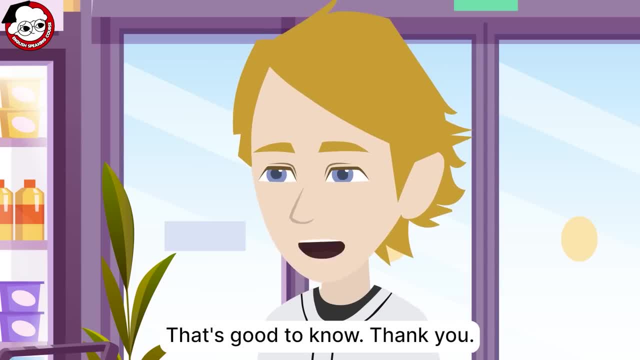 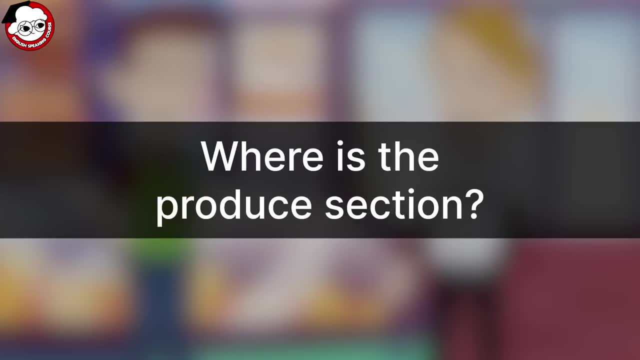 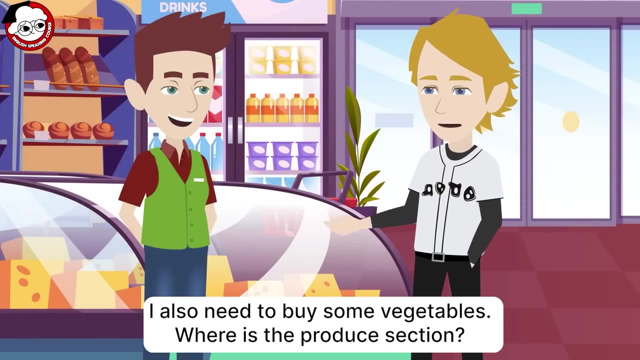 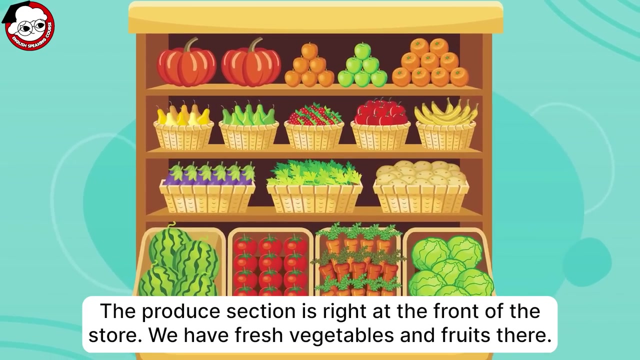 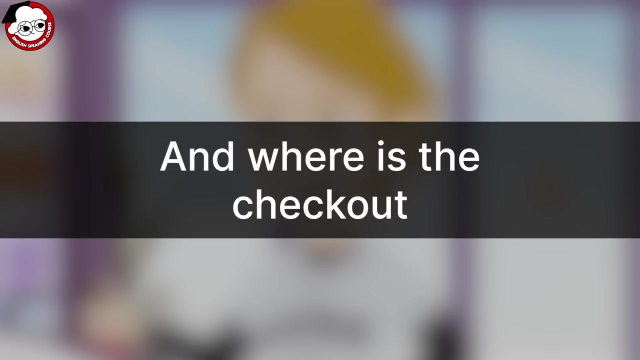 That's good to know. Thank you, I also need to buy some vegetables. Where is the produce section? The produce section is right at the front of the store. We have fresh vegetables and fruits there. I'll check it out. Perfect, I'll check it out. 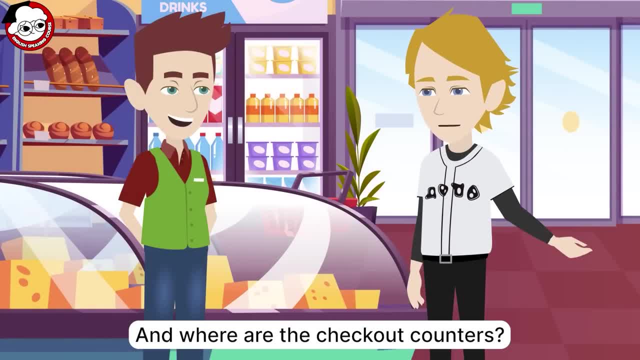 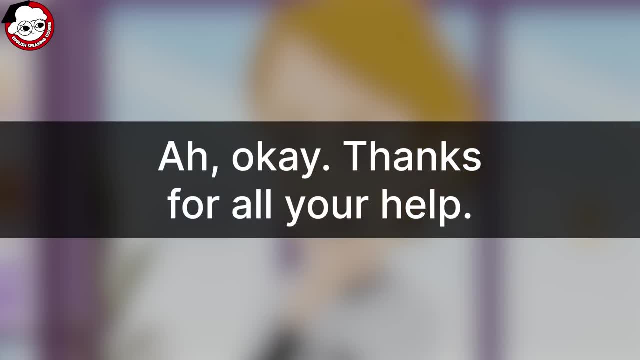 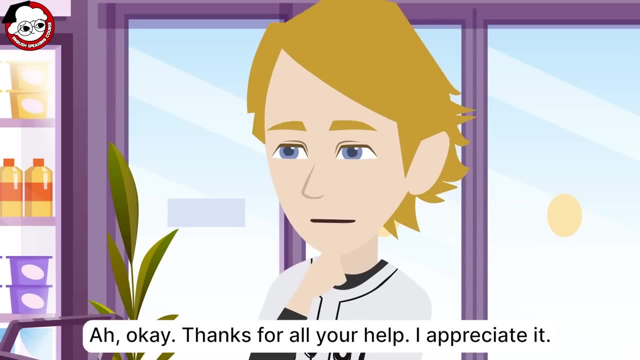 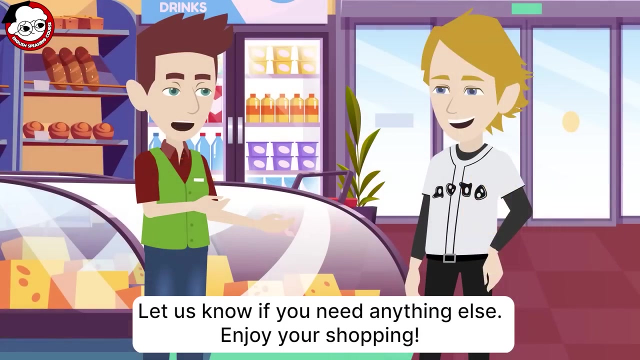 And where are the check-out counters? The check-out counters are near the exit. Ah, okay, Thanks for all your help. I appreciate it. You're welcome. You're welcome. Let us know if you need anything else. Enjoy your shopping. 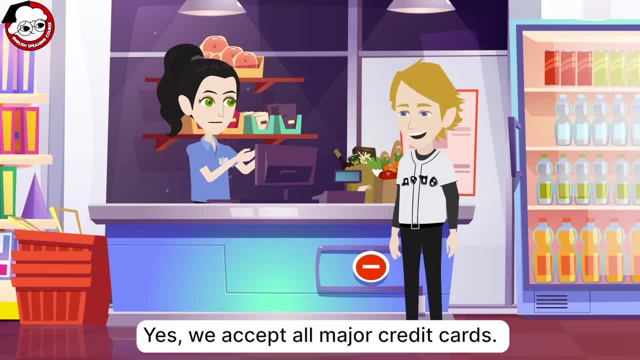 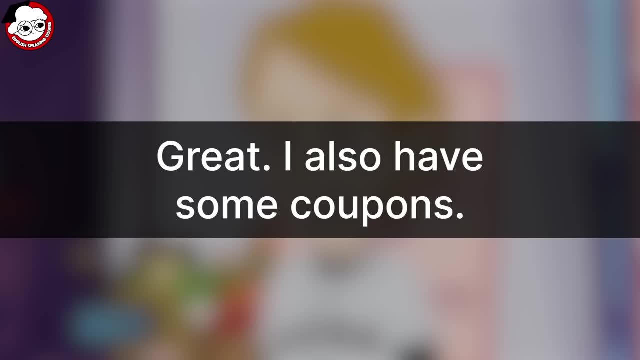 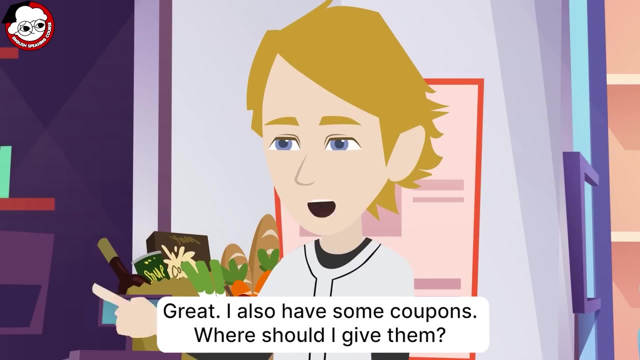 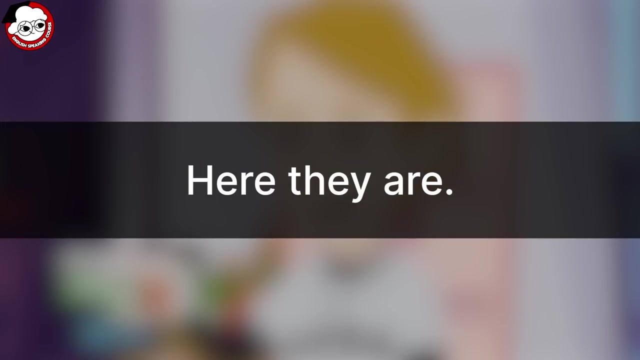 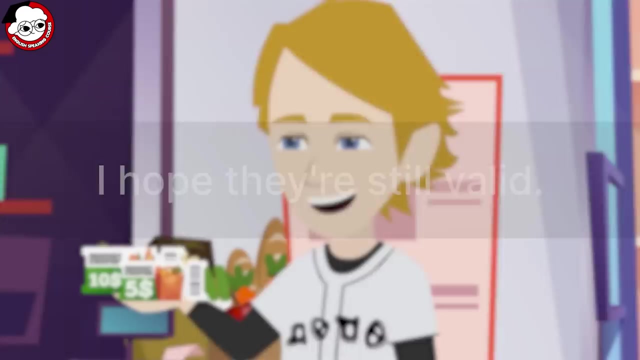 Can I pay with credit card here? Yes, we accept all major credit cards. Great, I also have some coupons. Where should I give them? You can hand them to me. I'll scan them with your items. Here they are. I hope they're still valid. 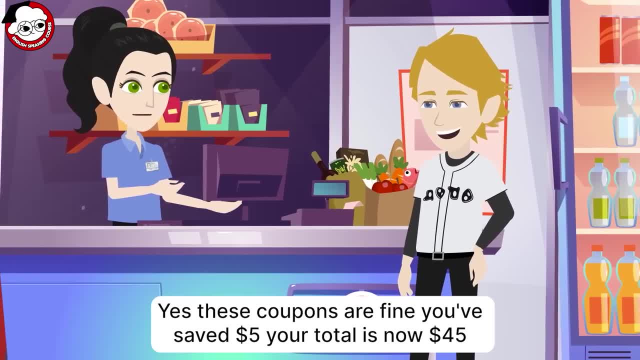 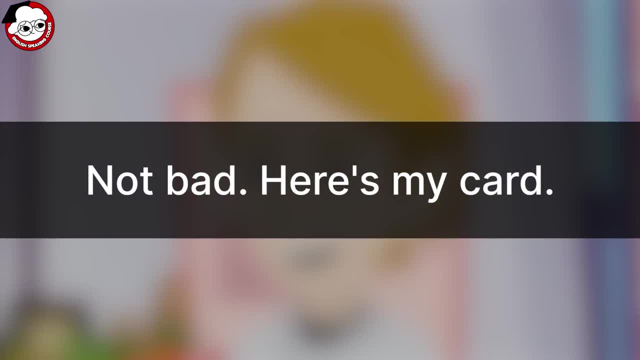 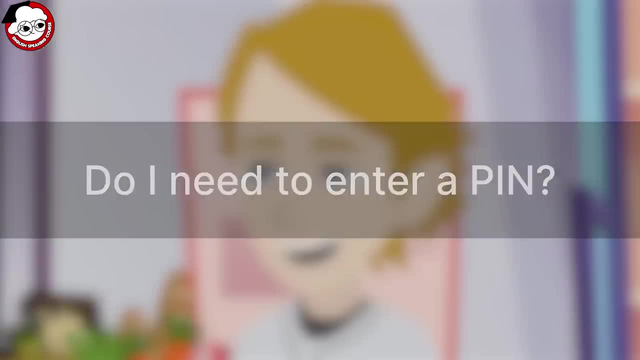 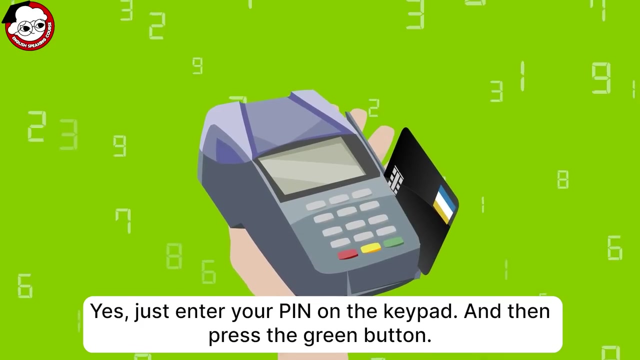 Let's check. Yes, these coupons are fine. You've saved $5.. Your total is now $45.. Not bad. Here's my card. Do I need to enter a PIN? Yes, Just enter your PIN on the keypad and then press the green button. 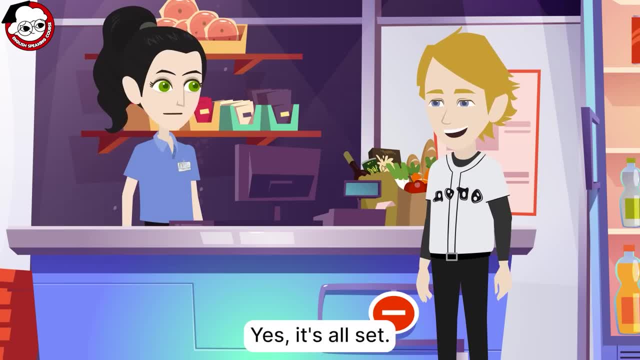 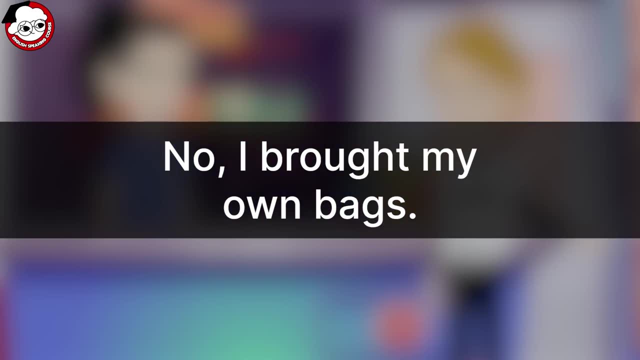 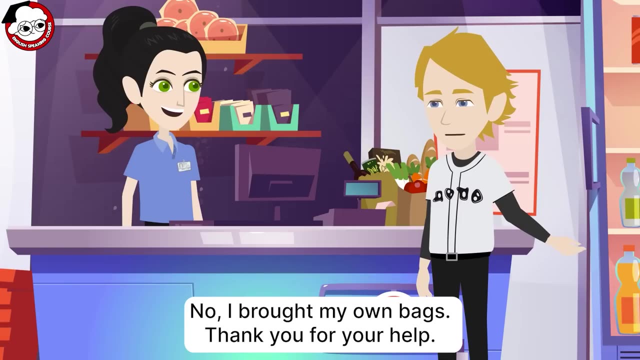 Done. Did it go through? Yes, it's all set. Here's your receipt and your card back. Do you need a bag? No, I brought my own bags. Thank you for your help. You're welcome. Have a great day. 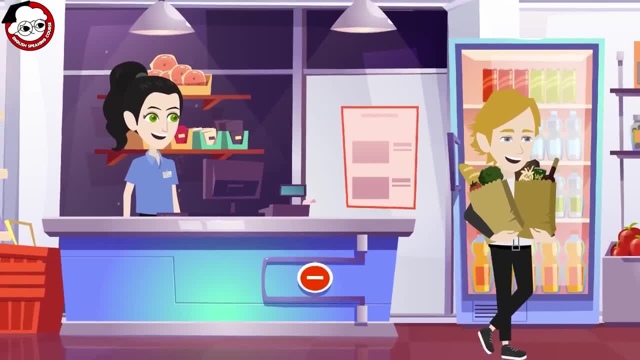 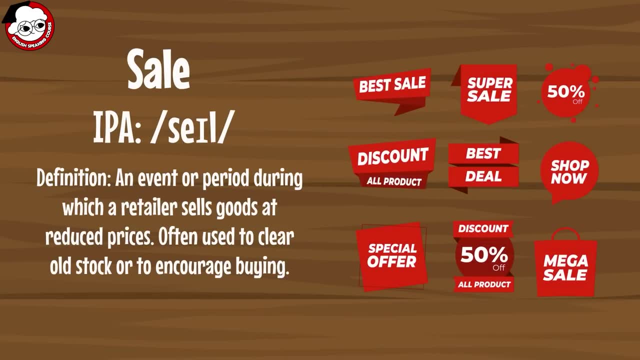 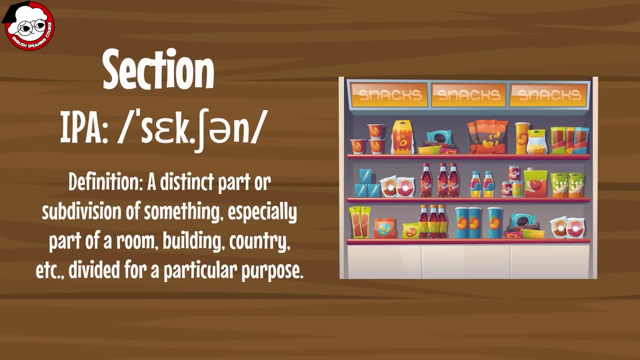 You're welcome. Have a great day reading. sale defini an event or period during which a retailer sells goods at reduced prices, often used to clear old stock or to encourage buying. section defini a distinct pair or subdivision of something, especially part of a room. 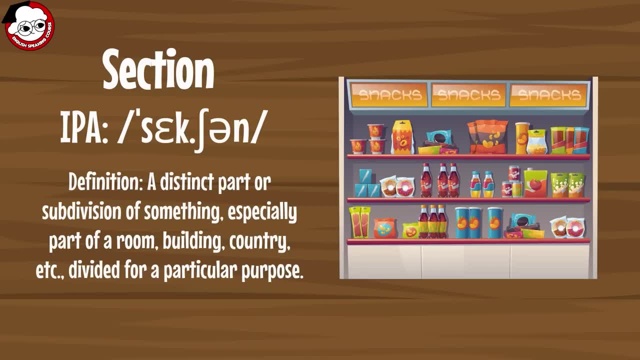 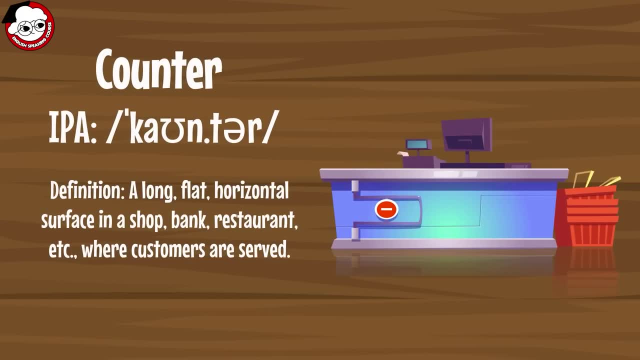 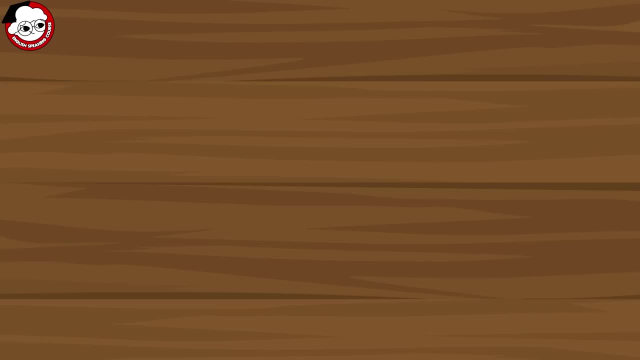 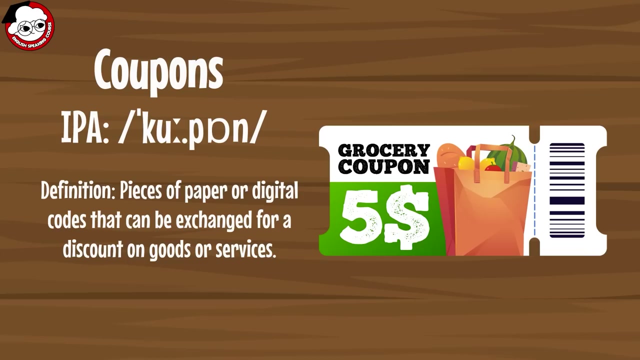 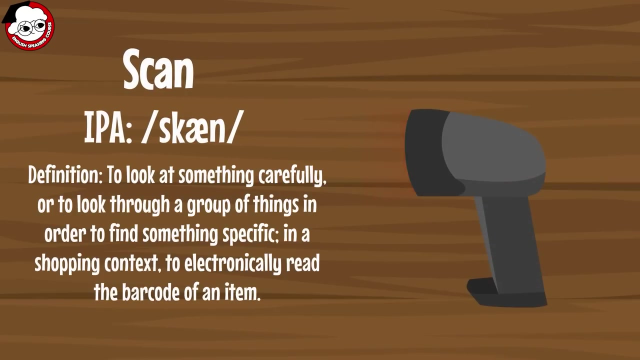 building, country, etc. for a particular purpose. counter definition: a long, flat horizontal surface in a shop, bank, restaurant, etc. where customers are served. coupons definition: pieces of paper or digital codes that can be exchanged for a discount on goods or services. scan definition to look at something. 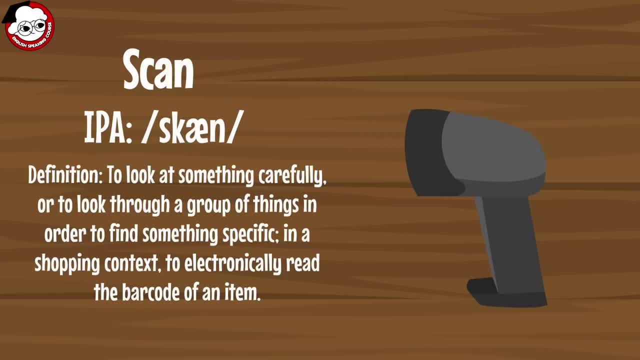 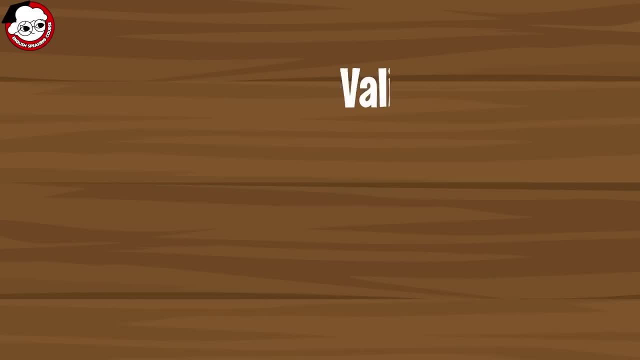 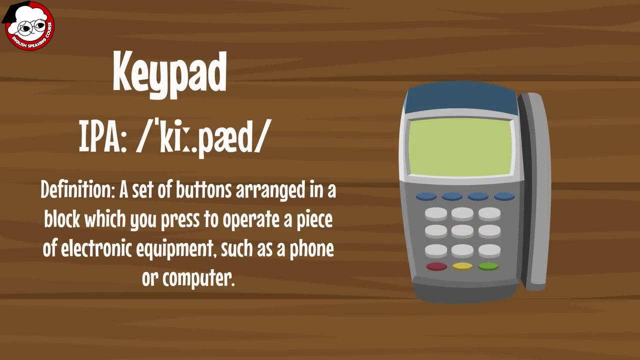 carefully, or to look through a group of things in order to find something specific in a shopping context. to electronically read the barcode off an item. valid definition: legally or officially acceptable based on truth or reason: having legal force. keypad definition: a set of buttons arranged in a block which would press to operate a piece of electronic equipment. such 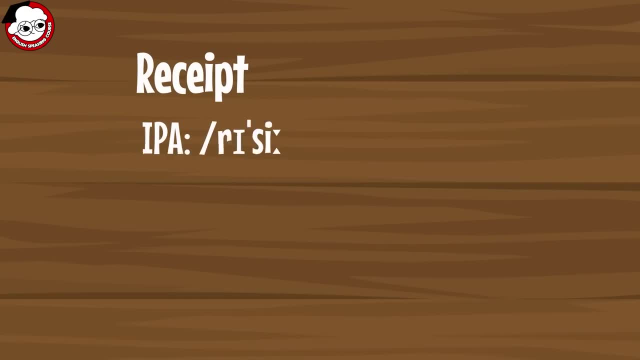 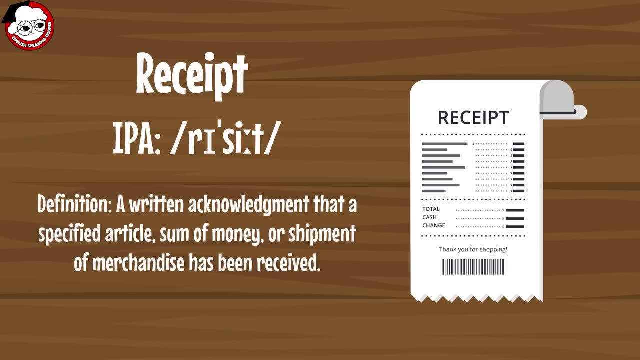 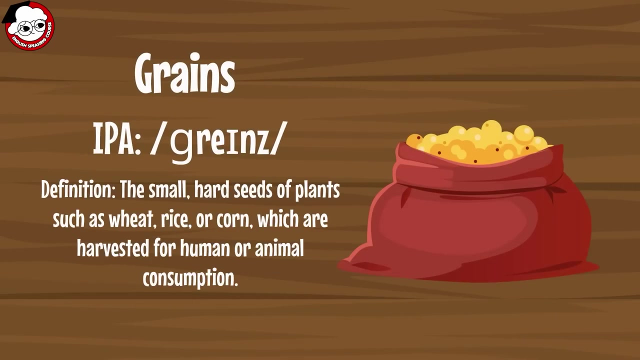 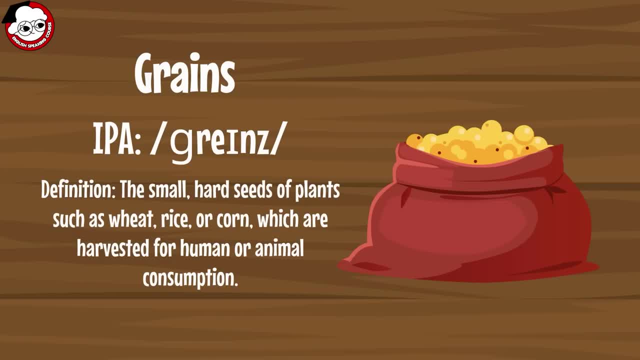 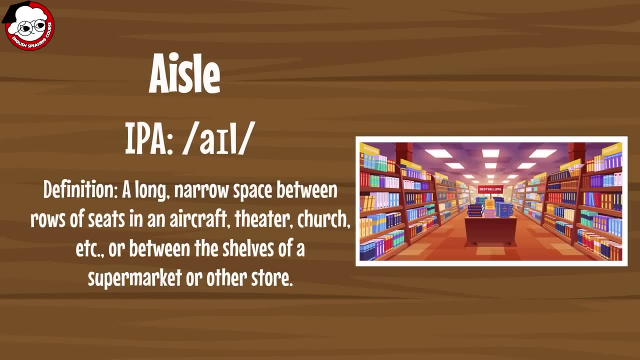 plants such as wheat, rice or corn which are harvested for human or animal consumption. aisle definition: a line of paper or document that is written on a piece of paper or document that is written on paper or on a freely available file. definition: a long, narrow space between rows of. 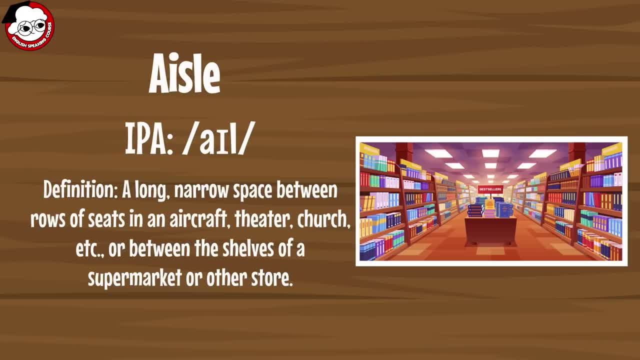 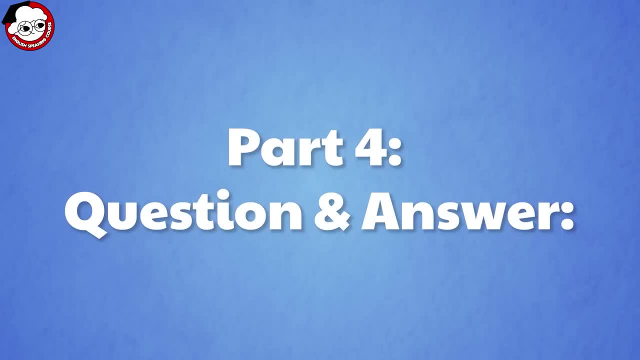 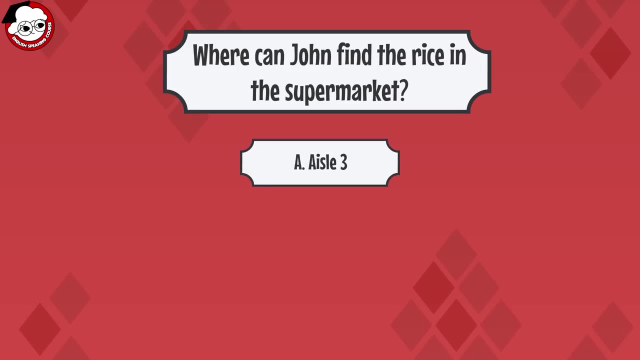 seats in an aircraft, theatre, church etc. or between the shelves of a supermarket or other store. where can John find the rice in the supermarket? a, isle 3b, isle 5c, at the front of the store. a? a, I'll see you later 17. 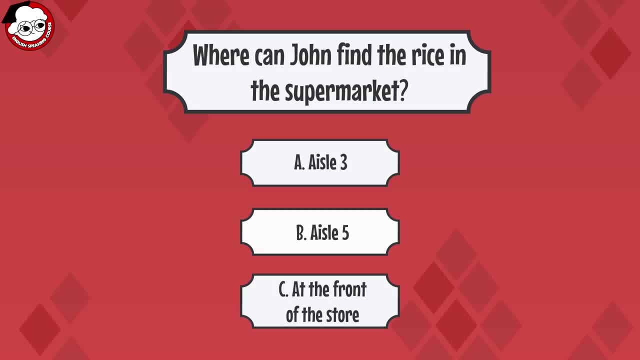 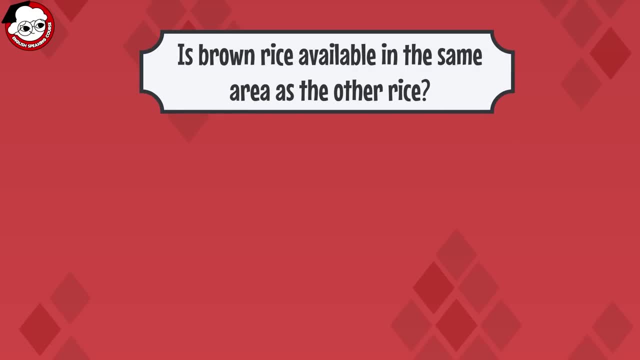 17, 17. you can and you can. you can, you and you can. The correct answer is B, aisle 5.. Is brown rice available in the same area as the other rice? A- yes, B no, C- not mentioned. 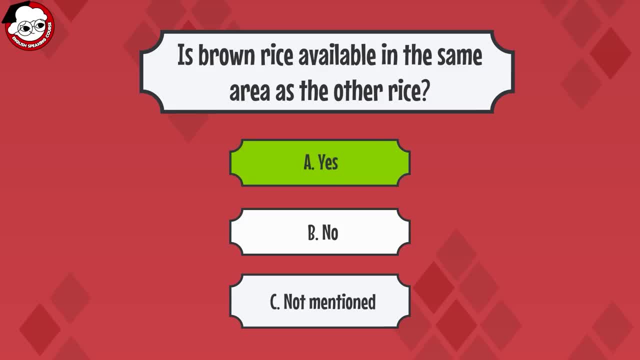 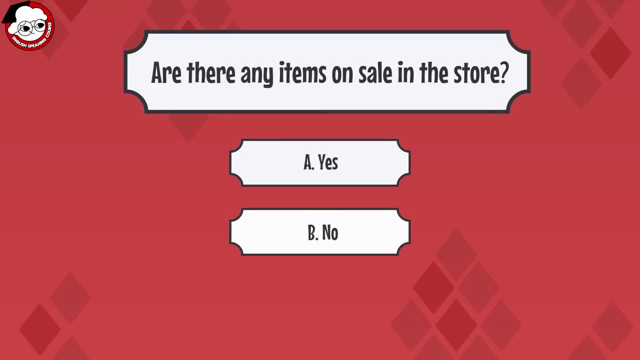 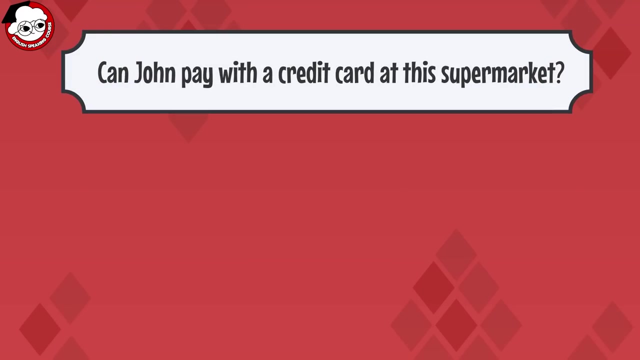 The correct answer is A- yes. Are there any items on sale in the store? The correct answer is A- yes. B, no, C, not specified. The correct answer is A- yes. Can John pay with a credit card at this supermarket?